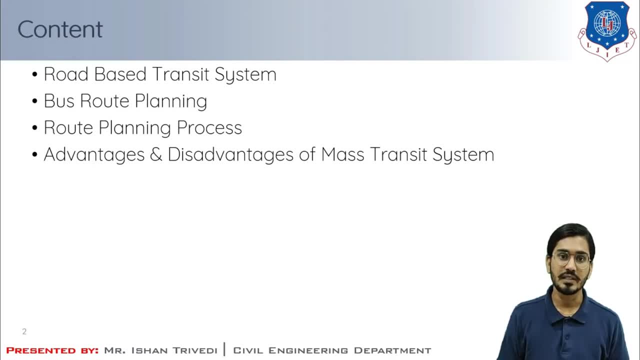 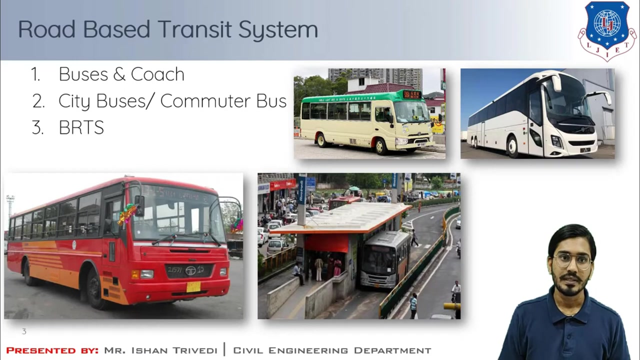 planning, their aims, necessity and factors, then bus route planning process and, at last, advantages and disadvantages of mass transit system. So let us start with the road based transit system. Road based transit system comprises with three major classification. These are buses and coaches, then city bus, or you can say commuter bus, and, at last, BR. 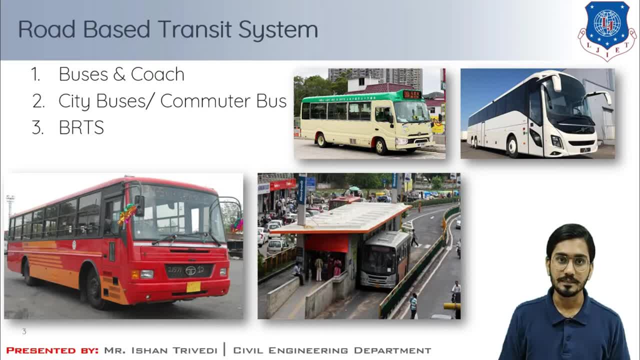 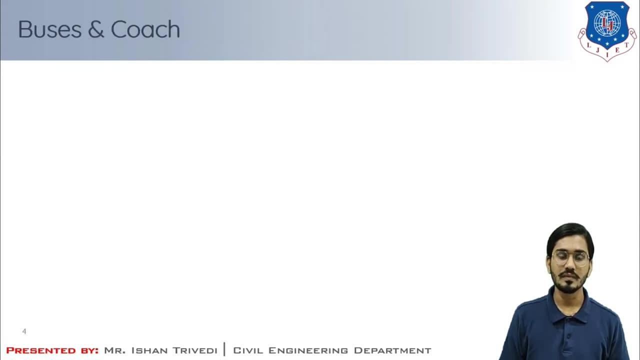 TS bus rapid transit system. Here you can see the photographs of bus transit, city buses and BR TS. So let us start with buses and coaches. Bus service uses the buses on conventional road to carry the numerous passengers on a shorter journey. These buses operate with: 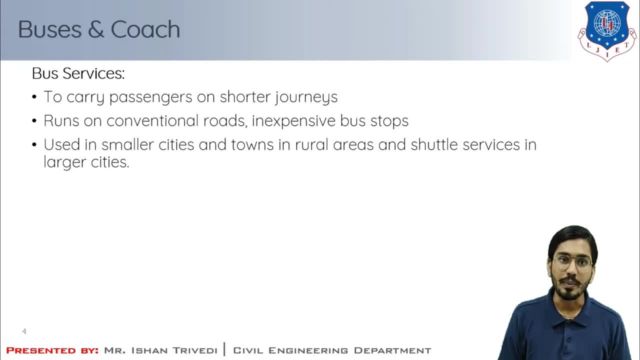 low capacity And it can operate on conventional road, as I said, with the relative inexpensive bus stops. There is not any major bus stop or any such facilities are there which serves the passengers. Buses are commonly used in the smaller cities or the town particularly. 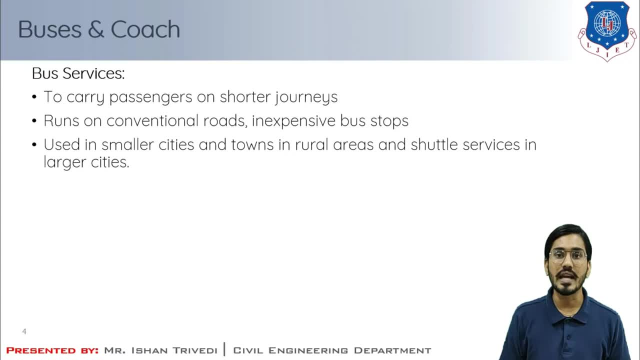 in the rural areas And these are used as a subtle services in large cities. Now, coach services, coach services use the coaches. It is a kind of a bus service which provides sleeping accommodation and it runs on longer distance. The vehicles are usually equipped with more comfortable settings and separate luggage compartment is there. And 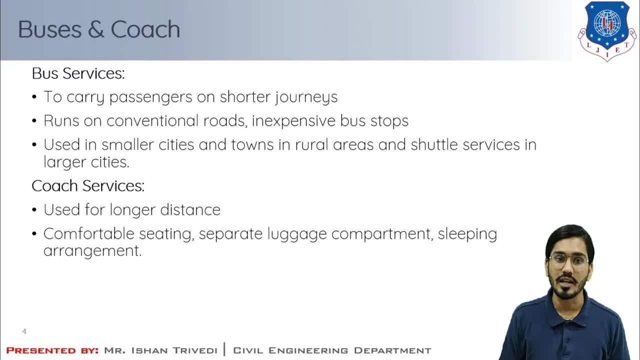 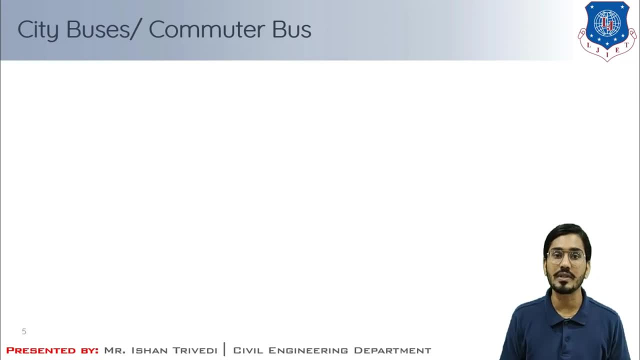 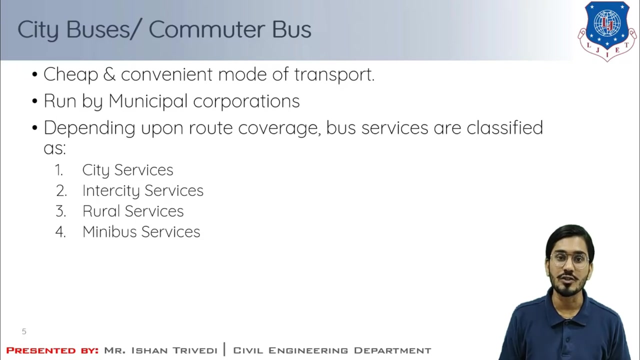 as I said, sometimes there are sleeping arrangement as well. Second is city buses, or you can say commuter buses. The city buses take up about 90% of the public transportation in Indian cities. This serves as a cheap and convenient mode of transportation for all the class of the. 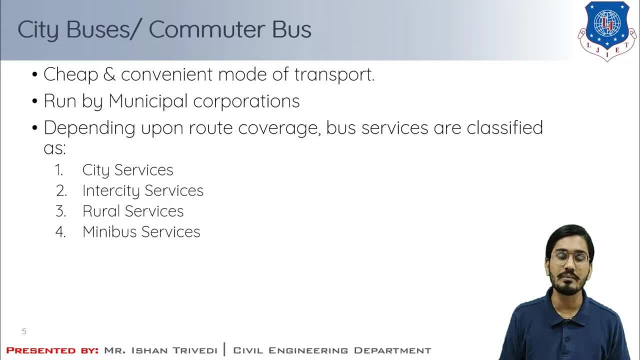 society. These services are mostly run by the municipal corporation. Bengaluru was the first city in India to introduce the Volvo city buses in 2006.. It was one of the first Indian cities to have an air conditioning bus stops located near the Gaban park. 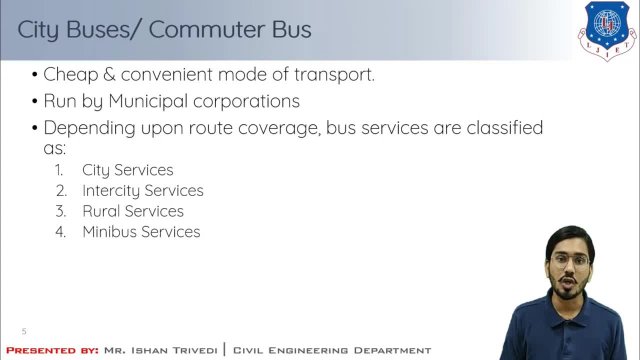 Hyderabad is also acknowledged for the single corporation having the largest fleet of the buses in the world, And there are many other cases in Indian cities, For example Hyderabad AMTS and Mumbai BMTS, which can be a part of study. You can refer these and have basic knowledge about these city buses and commuter buses. Depending on the route coverage, these bus services are of four types. These are city services, intercity services, rural services and minibus services. If I'm talking about city bus services, It covers the major route within the city limits. Then intercity, these services are providing the facilities between two major towns. 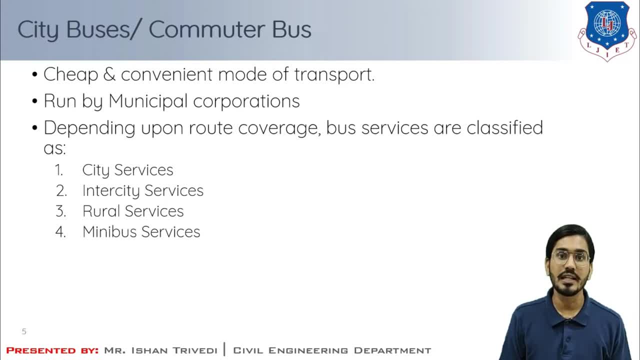 For example, Ahmedabad and Baroda. it runs the intercity buses as well. Then rural services: it connects the nearby villages with the cities and towns. You can say it as a rural transport or regional transport as well, But these services are limited. 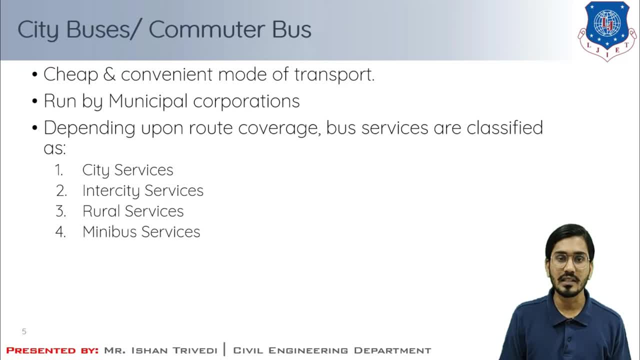 Up to the city limit and the nearness town of the city, Then minibus. Here the operation is resorted to when it is necessary to provide a bus connectivity on the routes which has less traffic demand and on route which are passing through narrow city streets. 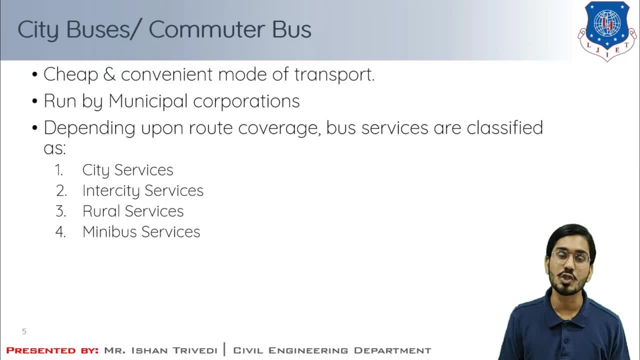 In some of the cases it runs as a feeder services to metro lines And in some of the cases it runs as a feeder services to metro lines, And in some of the cases it runs as a feeder services to metro lines And in some of the cases it runs as a feeder services to metro lines. 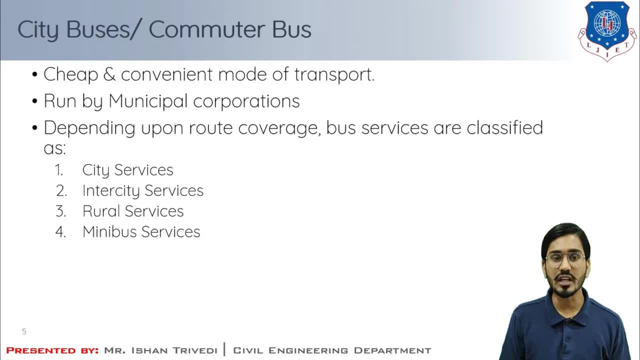 It runs as a feeder services to metro lines And in some of the cases it runs as a feeder services to metro lines And in some of the cases it runs as a feeder services to metro lines. If I'm talking about few advantages of this bus transport, then these buses can operate. 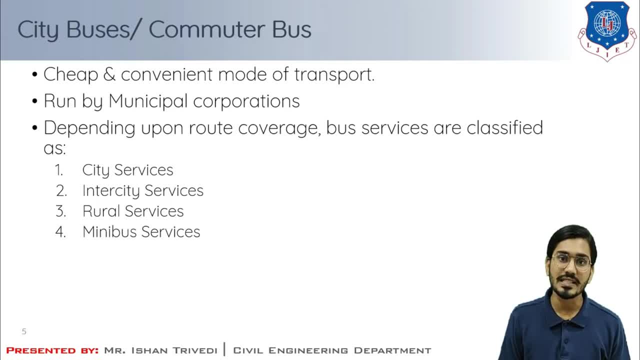 over the existing road system. Hence these bus can be implemented and expanded in a relatively shorter period of time. These bus routes are easily modified. Even you can modify the schedules very easily. It can be designed in such a way that it suits the demand. For example, in the morning peak the number of buses, or you can say frequencies of buses, are more than the afternoon time because it has lessen demand. Then buses can be used for charter and the other services. when not needed in the scheduled services, Buses can serve more diverse routes. 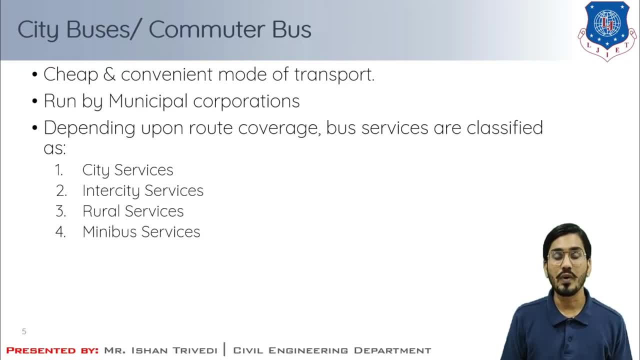 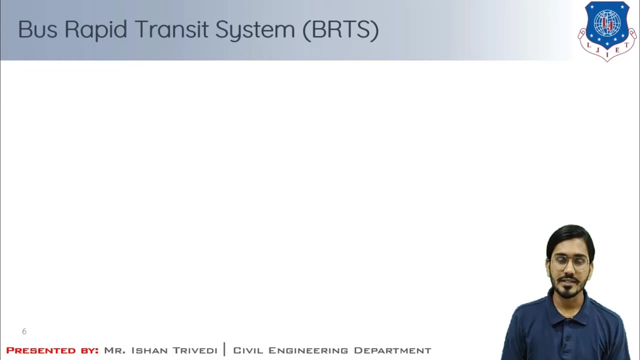 Low density travel pattern than fixed way system. So these are some of the important advantages of bus transport. Now BRTS: bus rapid transit system. In BRTS the buses move in a dedicated lanes at higher speed without any obstructions from vehicle crossing the links. 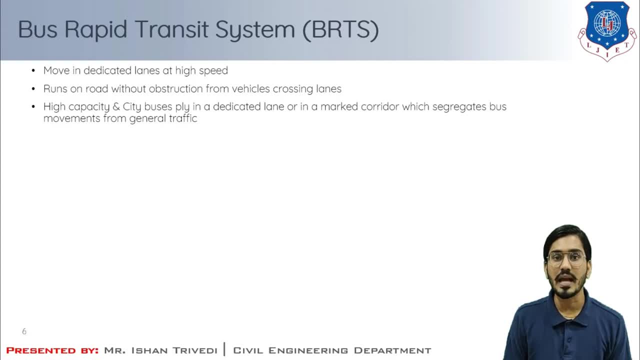 It has higher capacity And the normal city buses fly in a dedicated lane or in a marked corridor which segregates the bus movement from general traffic. Here, in Ahmedabad case, there is a separate corridor. in some of the cities in western countries where there is only a marked corridor, 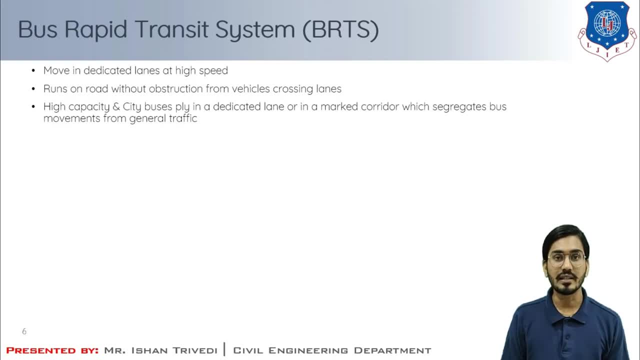 Here the segregation is been done by the writing that this particular lane is for the bus usage only. This BRTS concept has been carried out from the Bogota city. You can refer the BRTS system from Bogota as well. Delhi is one of the case, then Pimpri Chinchwar in Pune and Ahmedabad is one of the successful. 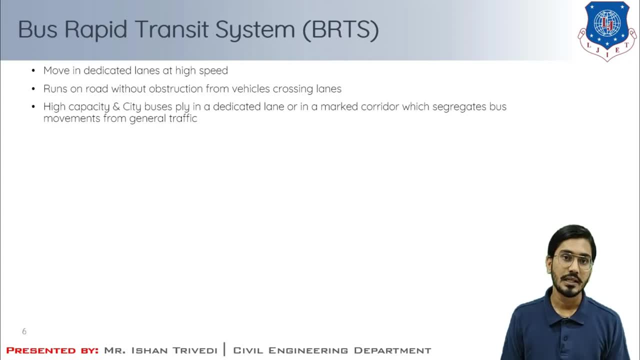 BRTS system. You can also refer the BRTS system of Surat city as well. If I am talking about the advantages, it has greater facilities in route options and the development, Then it has much faster development. then lower capital cost were dedicated in highway. 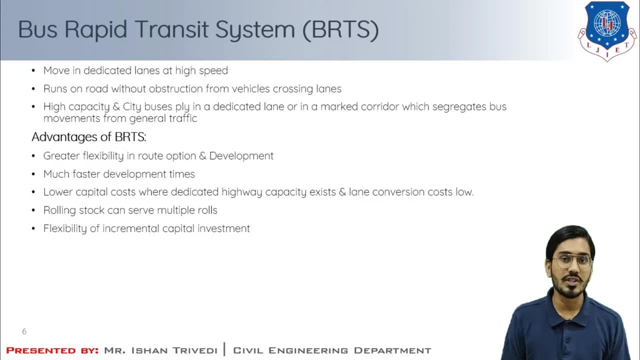 capacity exist and lane conversion cost is also low. Here the rolling stock can also serves multiple routes. Here the feasibility of incremental capital investment is also there. Now the disadvantage is there is a lack of availability of land for the dedicated lane in an urban area. 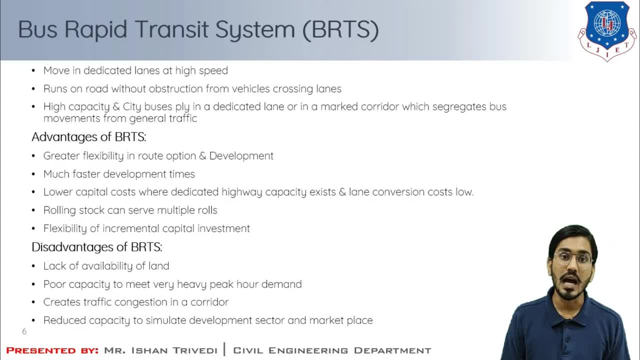 Poor capacity to meet very heavy peak are demand. due to limited bus carrying capacity, It creates traffic congestion in a corridor And, at last, it reduces the capacity to stimulate the development sector and the marketplace as well. So here these are the pros and cons of BRTS system. 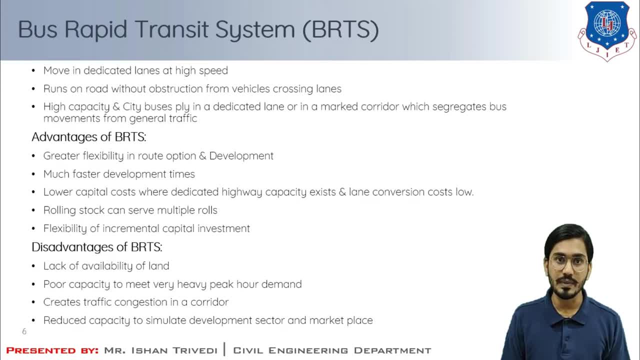 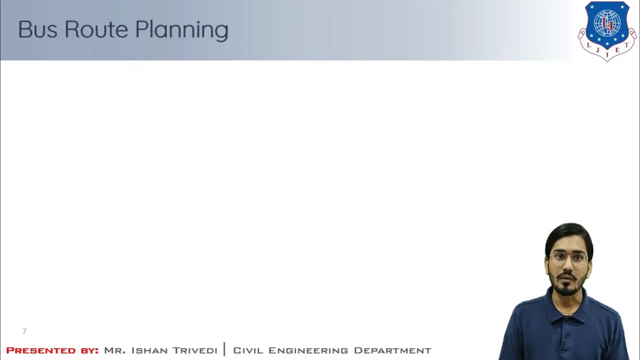 And you can refer the case studies of Indian cities: BRTS system. Now understand the concept of bus route planning. Transport by bus is the predominant mode of public transport in many Indian cities. China is one of the best example for this. In this metropolitan area there are about 80% of public transport trips are carried. 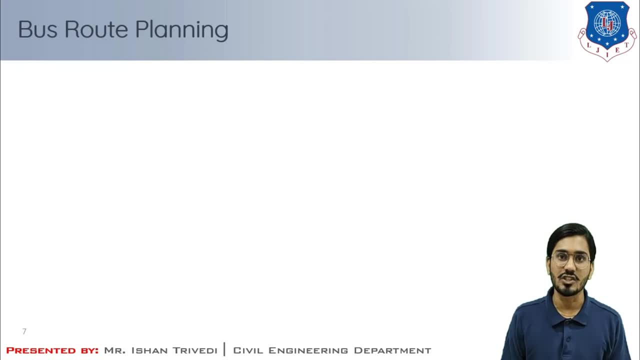 out by bus because of inadequate rail transit facilities. It depends upon the area. It depends upon the area bus route play a vital role in the efficient operation of the city bus system. Here the main aim of this bus route planning is about route planning to determine an acceptable 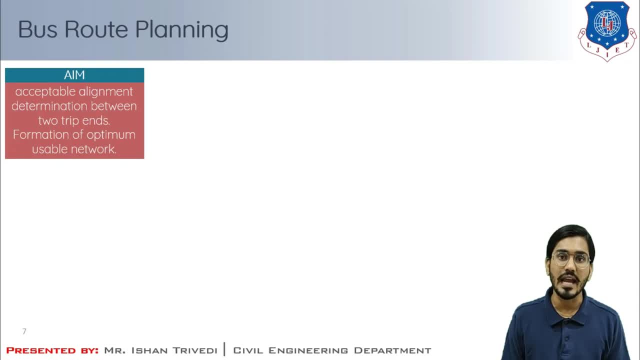 alignment for efficient, fast, reliable and portable bus operations between two trip ends. An additional aim is there: to form a network of such routes for urban area, which will lead to an optimal use of buses and other resources. Here we have need of the route planning. 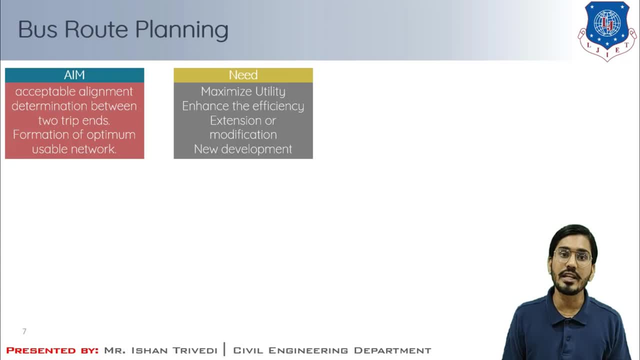 Here these situations are of: to maximize the utility of the existing fleet, to enhance the efficiency of existing road network, For the extension, or you can say modification, of these existing routes and for the new town under the development. If I am talking about the function of this bus route planning, then these are the collection. 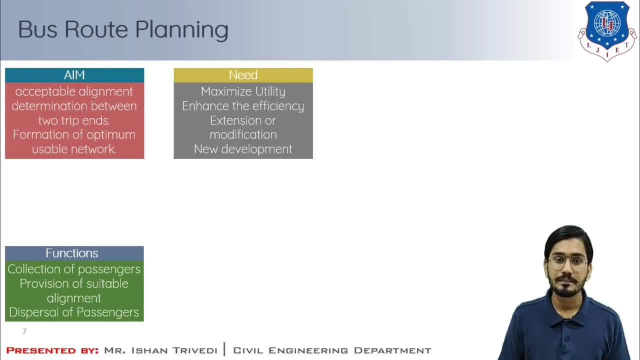 of passengers from dispersed residential areas, shopping areas and workplaces, Then there is a provision of suitable alignment for line haul between these origins and the destinations. Then dispersal of these passengers to their workplaces, shopping areas and residential areas: For any urban bus services it is feasible when the town should have minimum population. 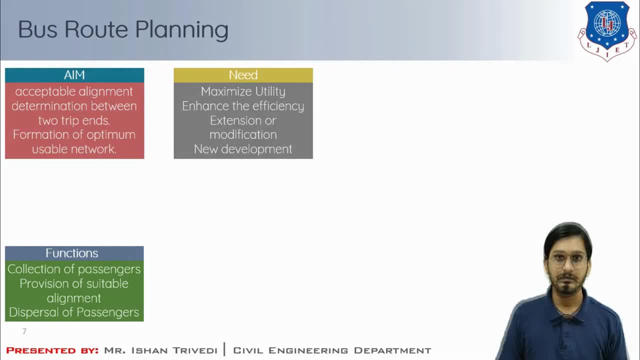 of 30,000.. Now, if I am talking about the passenger travel characteristics which are influencing this bus route planning, then that is also part of the discussion. The passenger demand over the period the onward and the return journeys are nearly equal: The passenger who are going from home to workplace and coming to workplace to home. this has to. 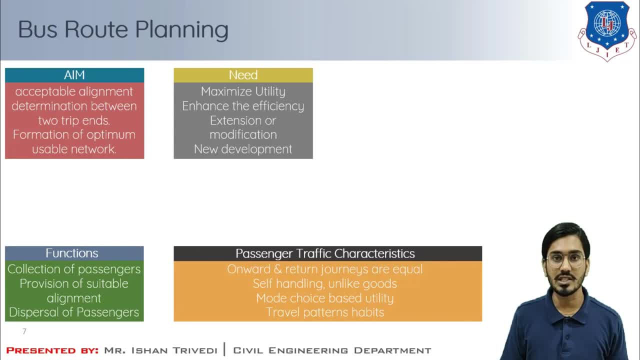 be in equal amount. So those who are using the bus transport for their up and down activities, it has to be in similar nature. Then the passenger handle themselves, unlike the goods which require handling and the delivery Passenger exercise choice of mode based on their perceived utility. 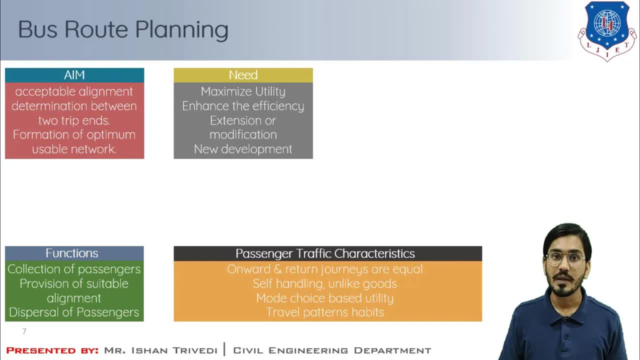 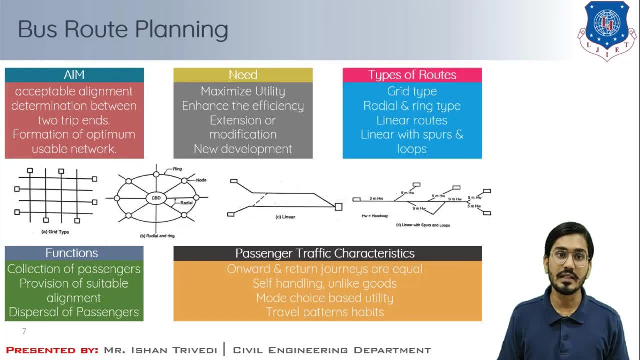 Passengers tends to form travel habits and they do not change their travel pattern easily. If I am talking about the types of routes, then these are of grid type, radial and ring type, Linear routes And linear with spurts and loops. So this is about bus route planning. 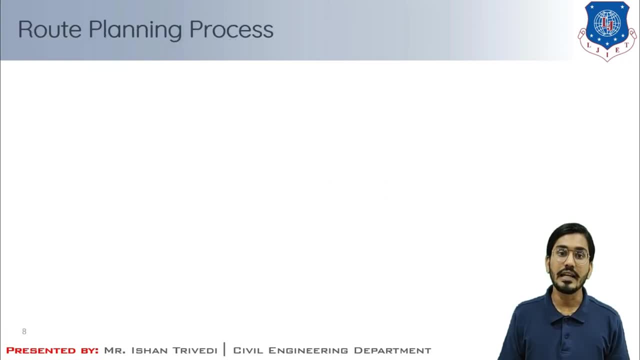 If I am talking about route planning process, then it comprises the four stages. First stage is the inventory of existing route network. We need to find out the where is the existing route network and, based on that, if there is any change in this particular route network. 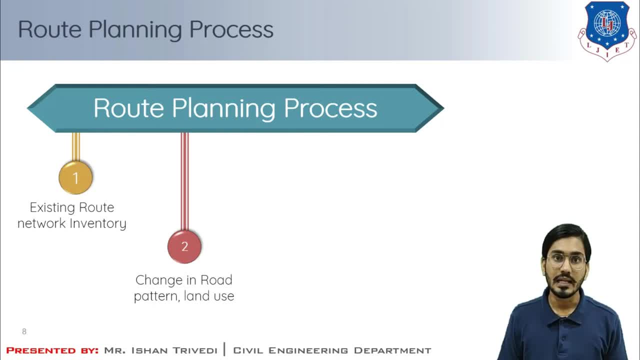 And their particular route from the different areas, then you can change it, even for the future road building and the land use form. you may extend those routes if so required. Then the origin destination pairs of the present and the projected routes are also in study date, which is part of route planning process. 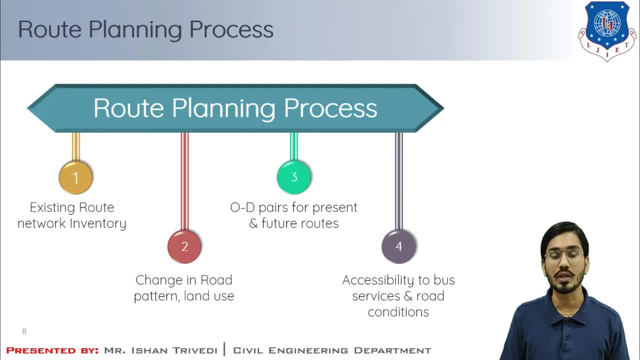 Then, at last, the accessibility to bus services and the road conditions Here. this bus services means the different locations of depots and the bus stations as well, and the system- this system runs on the road- that also affect means the road conditions. So this is about bus route planning and route planning processes. 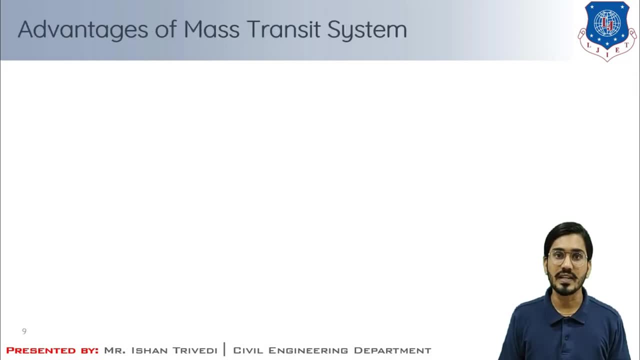 Now understand the advantages of the mass transit system. Here There are Few Impacts of the these mass transit system. Let us study these impacts. First is environmental impacts. Mass transit is believed to be more environmental friendly than the other mode of public transportation. 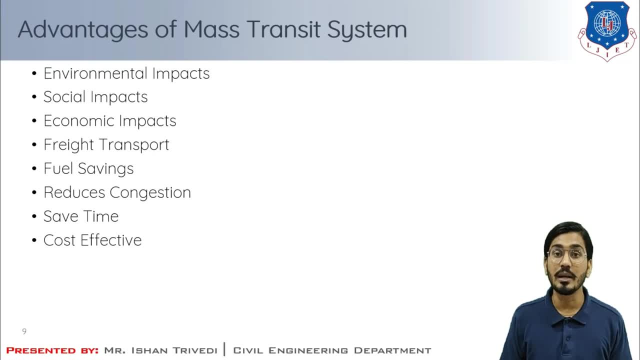 facilities. Mass transit reduces the number of cars on the roads, which in turn reduces the air pollution. Public vehicle releases less toxic gases like hydrogen, Like hydrogen, like carbon monoxide, which is major air pollutant. then if i'm talking about the social impacts, 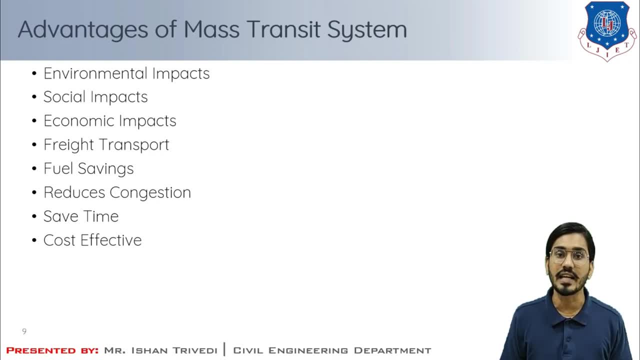 then all the members of the society, irrespective of their culture, financial status, religion or the cars are able to travel, which enhance the social integrity of the country, and the necessity of driving license is also eliminated. then, if i'm talking about the economic impacts, it results in the increasing the business, commercial development and thus it offers considerable savings in the 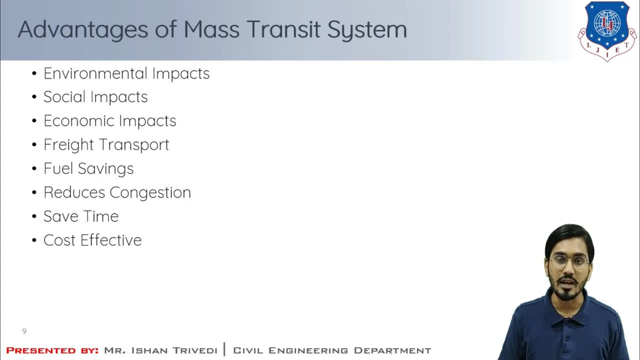 labor, material and the energy over a private transit system. then the freight transport. it allows higher amount of load to be transported to far away destination in the lesser tech than fuel savings. because of their large capacity, offering them to carry higher efficient engines, they also help in fuel savings as well. some of them are using the electric. 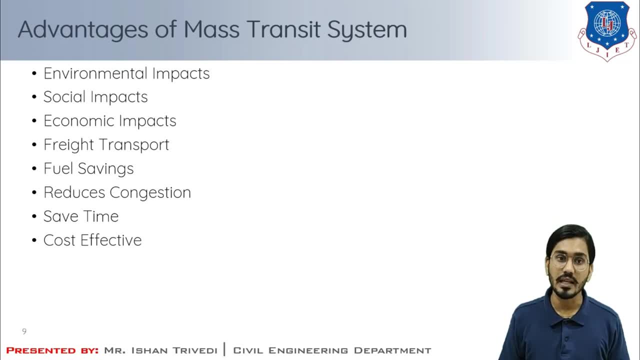 cable, so there is considerable saving in the fuel as well- then reduces the traffic congestion. it reduces the number of vehicles on the roads by providing large number of capacity vehicles which carries higher number of passengers, and thus eliminating the congestion on the roads, then saving in the time. mass transit reduces the travel time to a great extent. 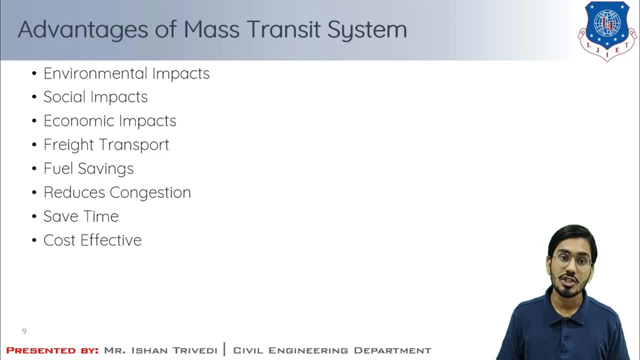 as it moves at high speed and stop only at specific spots. if i'm talking about a metro station, it has been provided at an average distance of 1 to 1.5 kilometer. if i'm talking about brts, the stoppage are of nearly 800 meters and the city bus services the average stop in amgabadi.